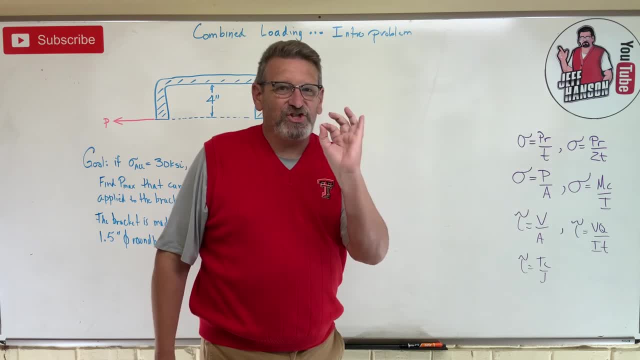 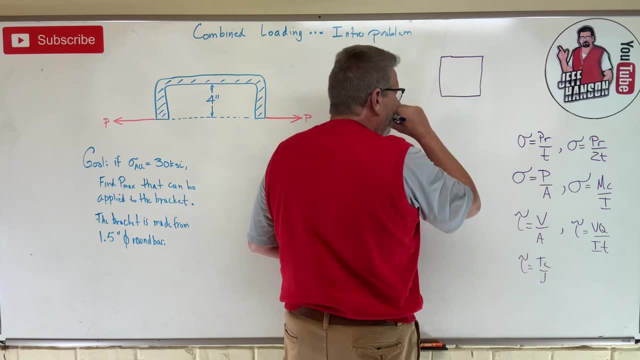 look over here. What we're going to be looking at is the state of stress, okay. And when I say state of stress, here is a stress element, a little piece of material, a little microscopic piece of material. We said, okay, what's going on with that little piece of material, right? 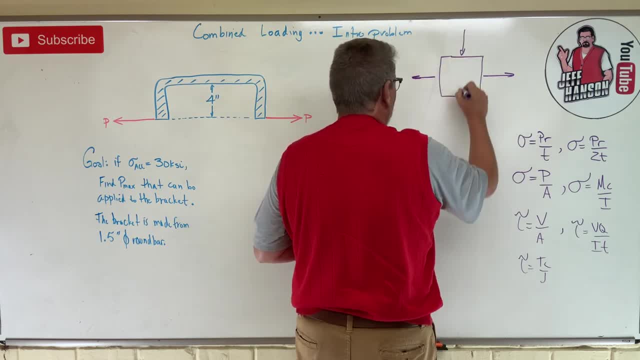 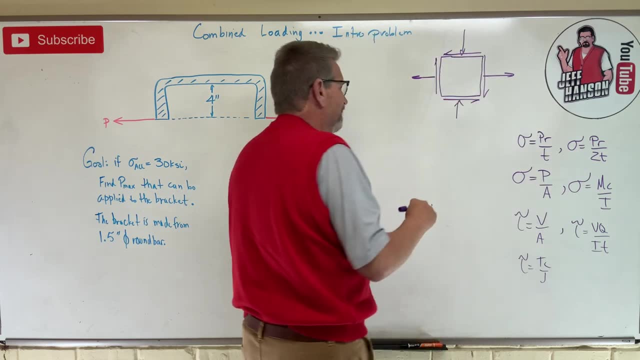 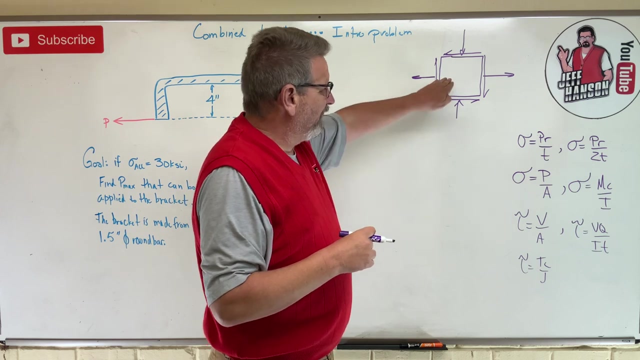 He's being stretched, he's being compressed, he's being ripped and torn and right he's got sheer stress, he's got normal stress and all kinds of little things On that little piece of material right, And we're going to be interested in what is going on on that. 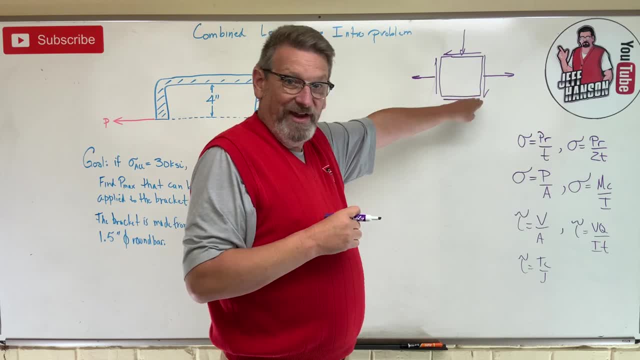 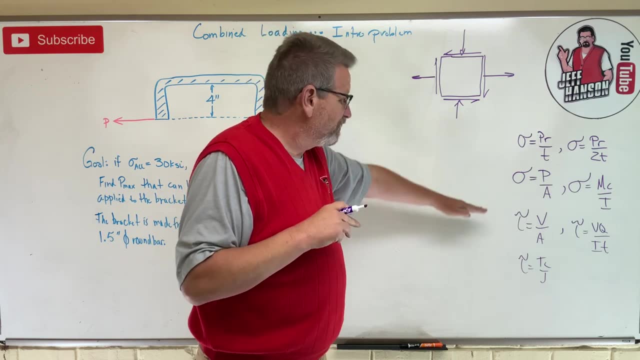 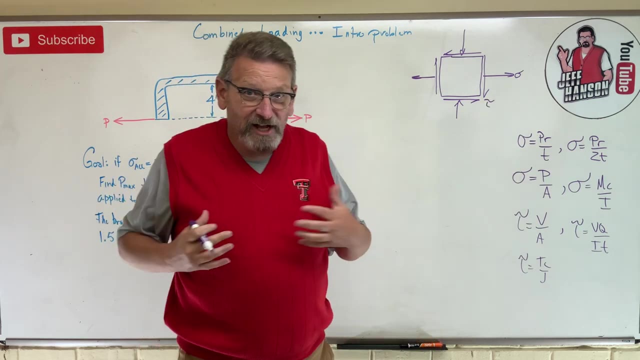 piece of material, at a particular point, on a part, and the stress, which could be sigma stress or tau stress- here's our sigma stress over here, here's our tau stress down there- could be caused by lots of different things, right? Who causes normal stress? Who causes sigma stress? Well, 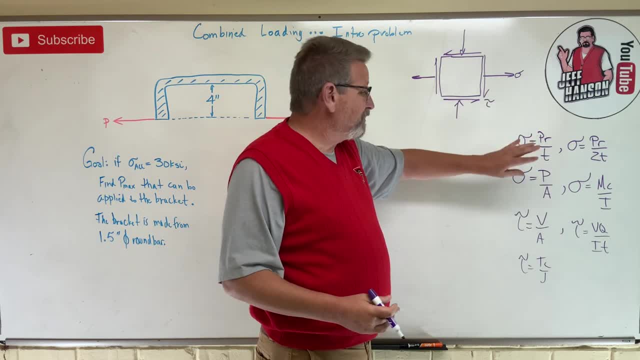 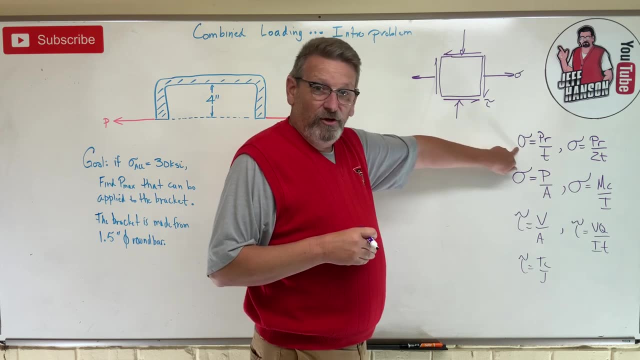 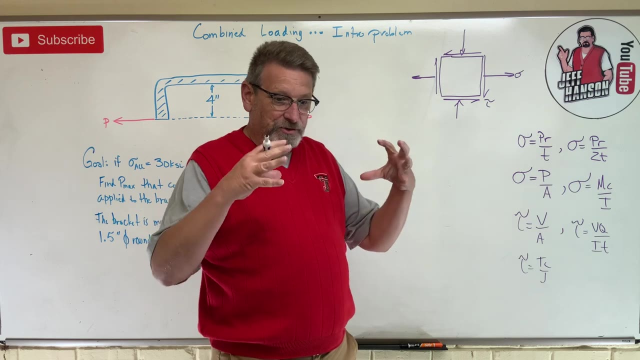 if it's on. if that little piece of material is on a pressure vessel, right A thin wall pressure vessel- we just covered it with these equations, didn't we- Then that could be caused by hoop stress or longitudinal stress. What if I have a pressure tank and also, at the same time, somebody's? 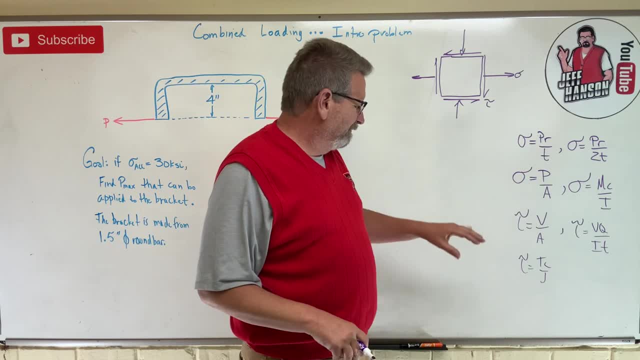 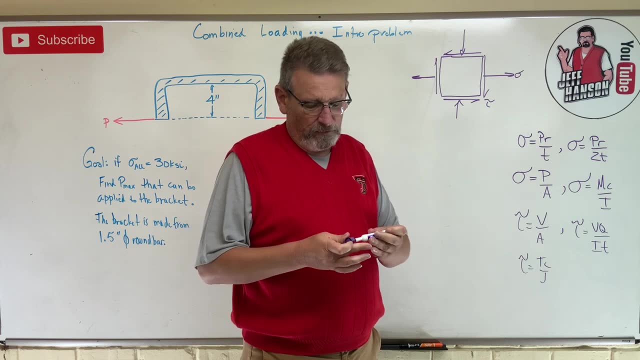 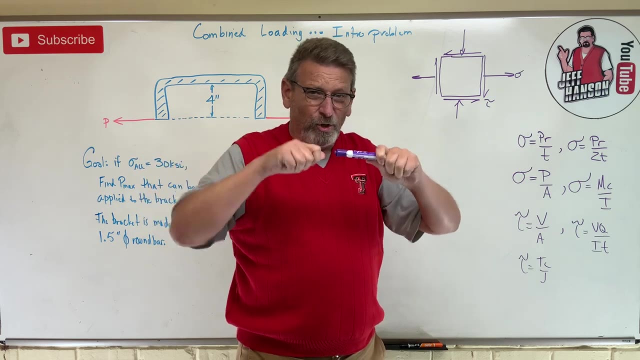 stretching it right, Just pulling on it. Well then, there's an additional stress from just P over A, from normal stress. Remember, normal stress is pushing on it or pulling on it right, Making it longer or shorter kind of stress. 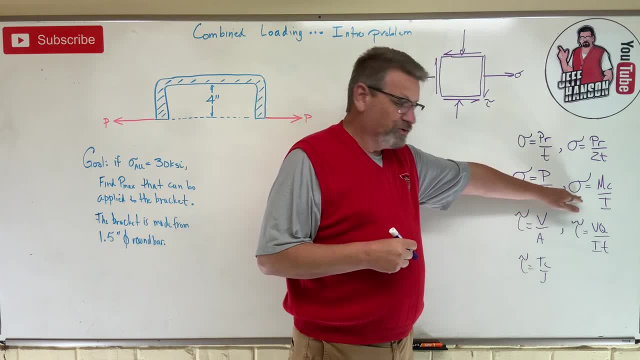 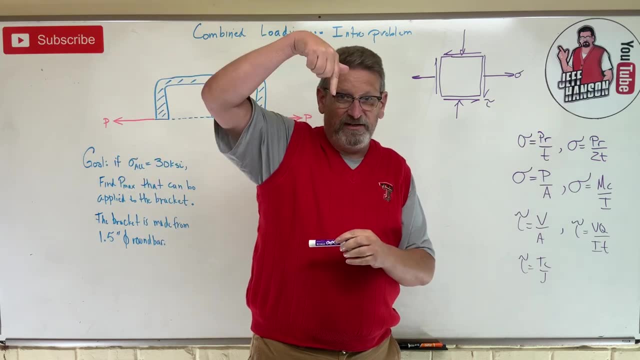 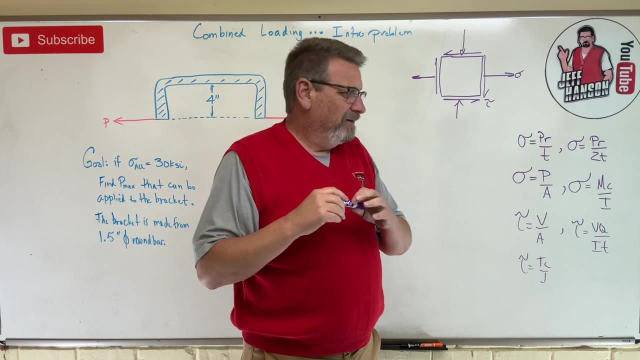 P over A stress, Or stress could be coming from if there's a load on it right And it's causing it to deflect right The top of it's in tension or in compression, the bottom of it's in tension as it gets bent right, And so that's called bending stress. We have our flexion. 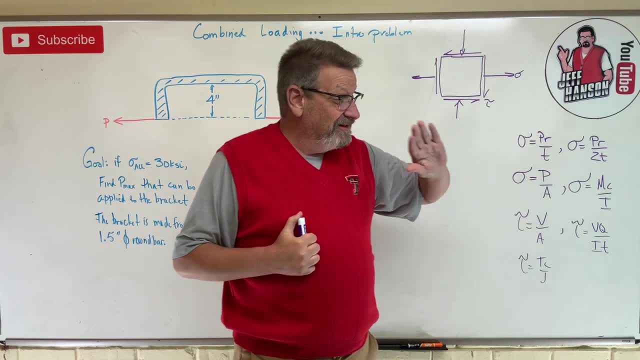 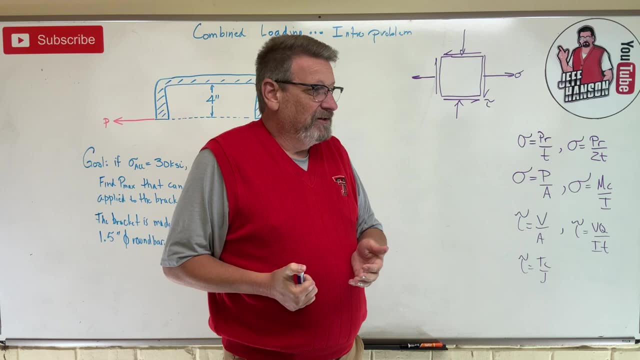 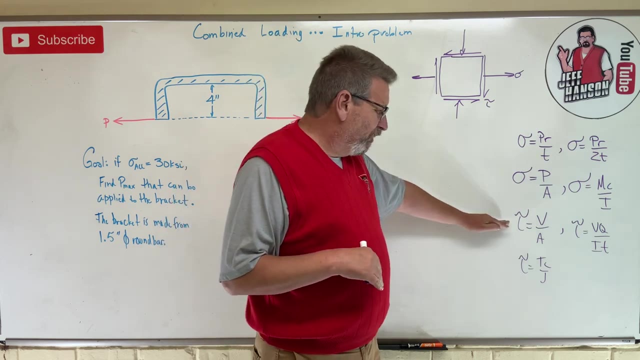 we have our pressure formula, MC over I, to calculate sigma stress from beam bending. So sigma stress can come from a lot of different places, right, And guess what? They're all sigma stress, They're all the same thing. and they add together: Oh my goodness, Or shear stress, Same. 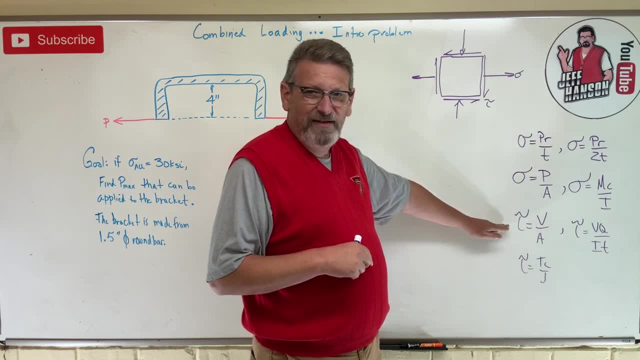 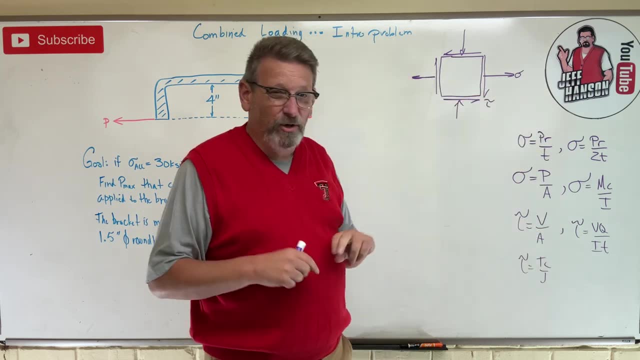 thing, Shear stress can be caused by what V over A- Now V over A is average shear stress. We looked at VQ over IT And since we're looking at a particular particular point in some material, VQ over IT, remember, is the stress at a particular point. 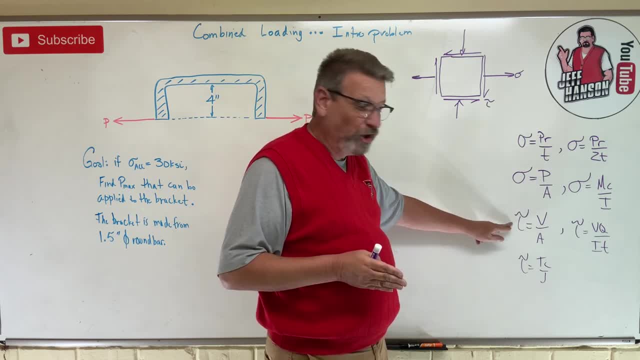 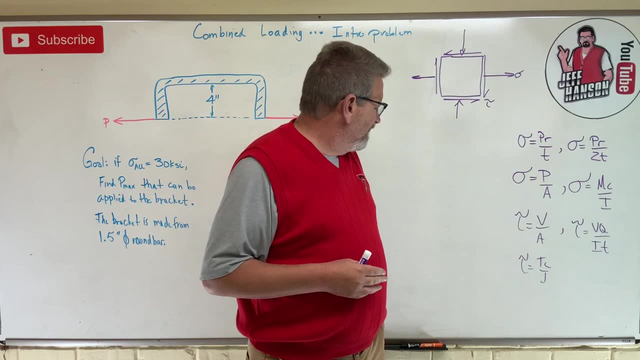 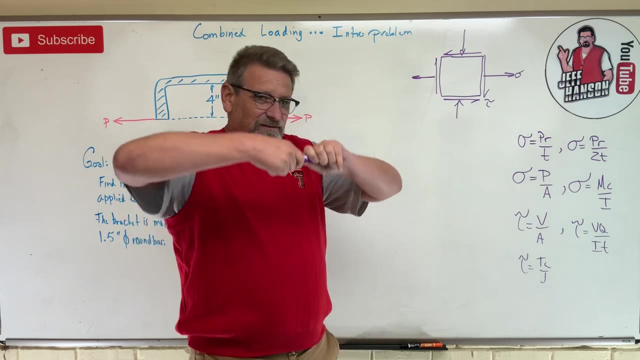 where V over A is the average over the whole surface. So probably we're going to be using VQ over IT, a lot Transverse shear, as well as TC over J. Now that's what kind of shear is that? That's torsional shear, right? That's from twisting. So if I'm twisting something, 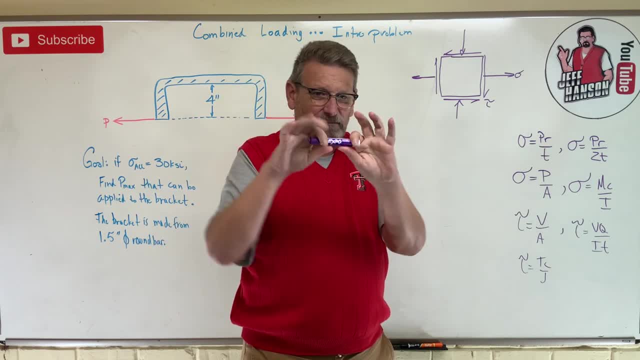 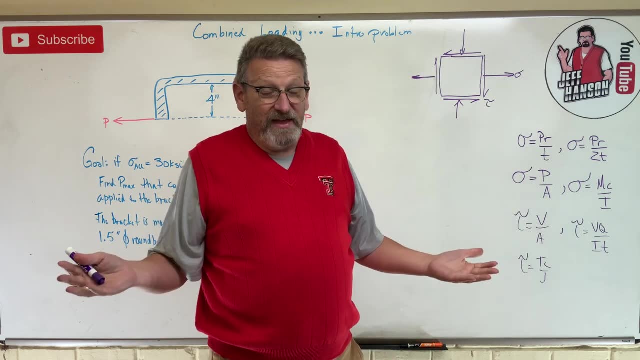 I could be tearing it And then I could as I bend it. maybe I'm bending and twisting at the same time. I got both of those things going on at the same time. They add together or they subtract one from the other and we're going to. 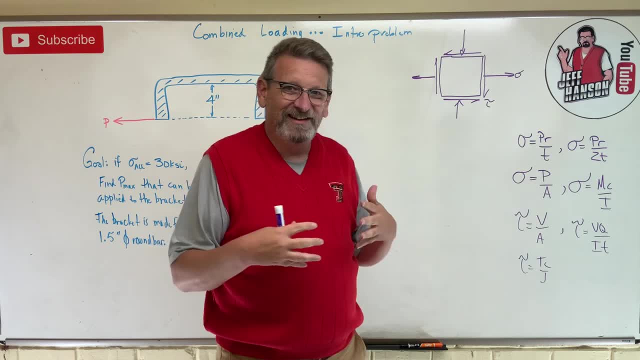 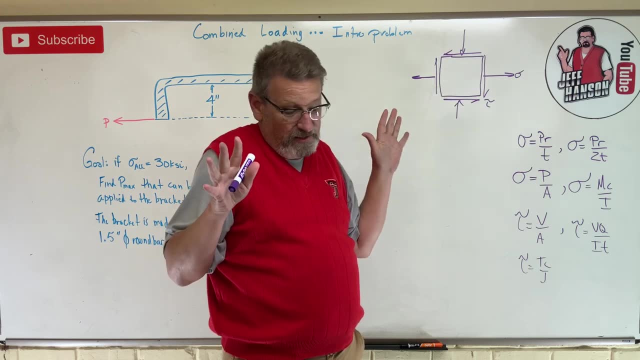 have to combine them, combined loads, and find out what is the state of stress at some point in the material. That's what we're doing. okay, It's going to get confusing y'all, because all the problems so far have just had one kind of thing happen. 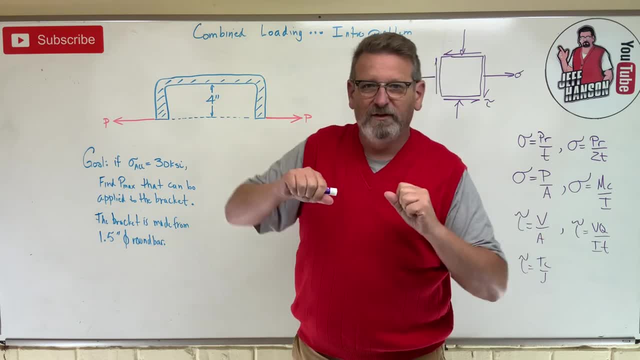 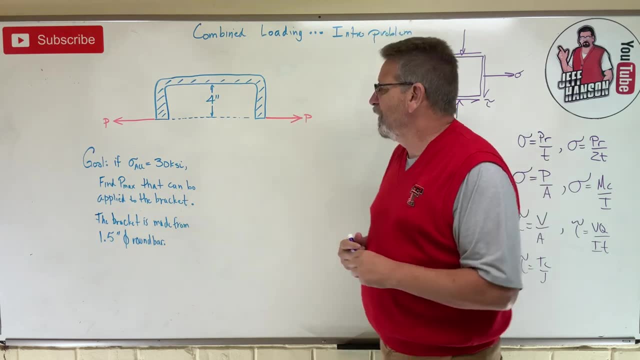 They're getting stretched, they're getting compressed, they're getting bent. But now they're getting bent, stretched, compressed, under pressure- you know what in the world? So hang on, it's going to be all right, I'm going to get you there, It's going to be all right. 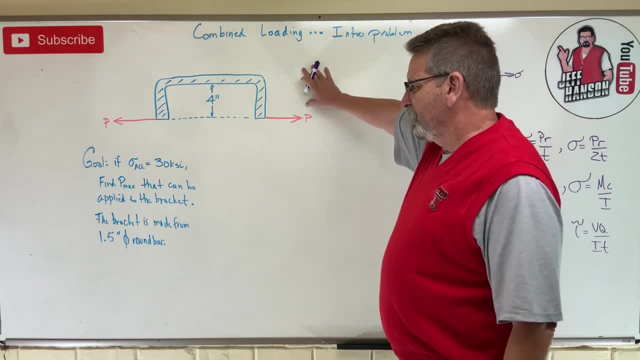 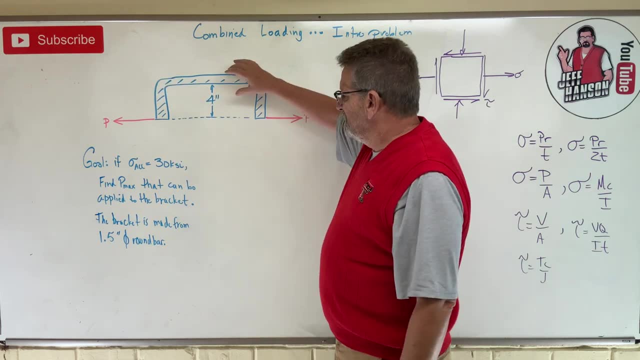 Okay. so here we go, Combined load. We're going to start off a little easy one, okay. So we have this little bracket- Maybe this is a handle on your barbecue grill or something right- And what happens here on this bracket is made out of an inch and a half diameter. 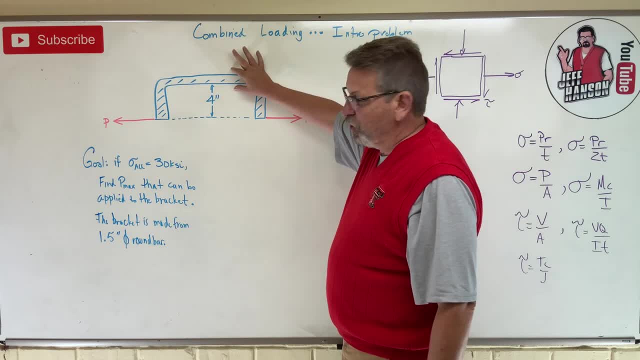 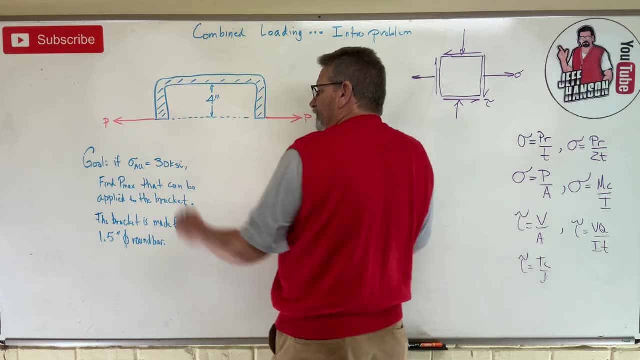 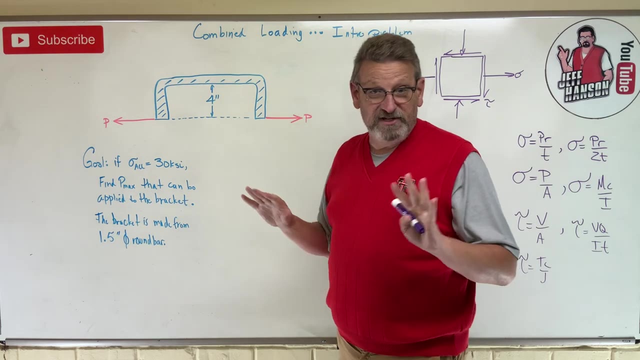 round bar. okay, So one and a half inch diameter. okay, It's bent. And then it has some. for some reason it's got force on the end of it pulling on it, right? If sigma allowable is 30 ksi, okay, Sigma allowable, that means that's all it can take before it deforms. 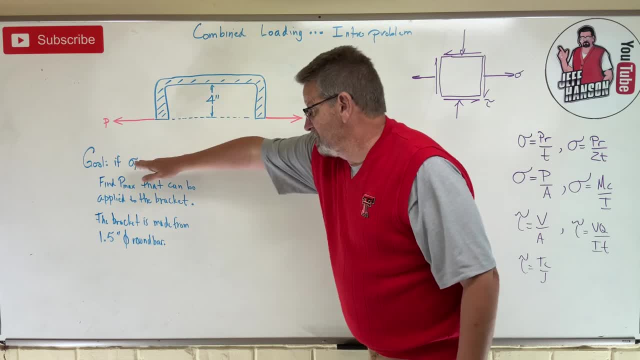 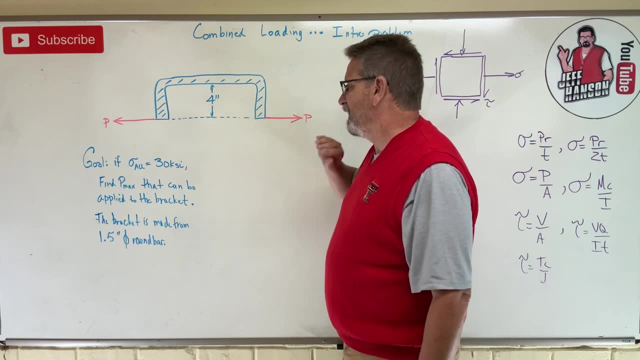 right, That's probably like probably another way to say that is, yield stress is 30 ksi. We learned about that too. didn't we Find Pmax so that they It can be applied to that bracket without causing it to fail? This is our failure point. 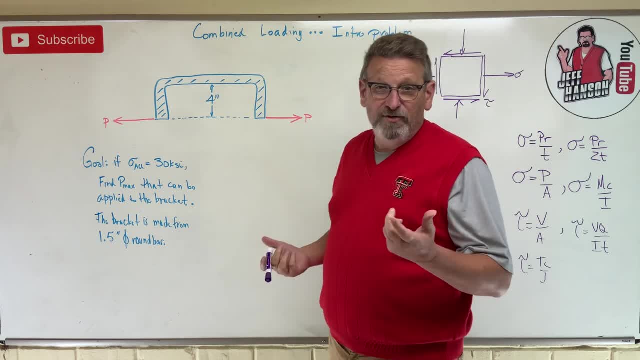 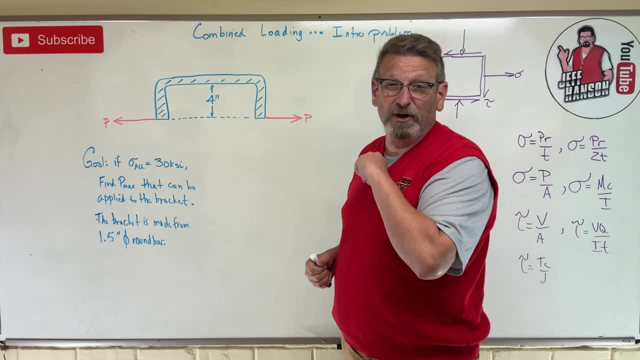 okay. So how big is P Now? how much force is on that bracket? How many of you out there would say it's 2P? How many of you out there would say it's 1P? If that's confusing to. 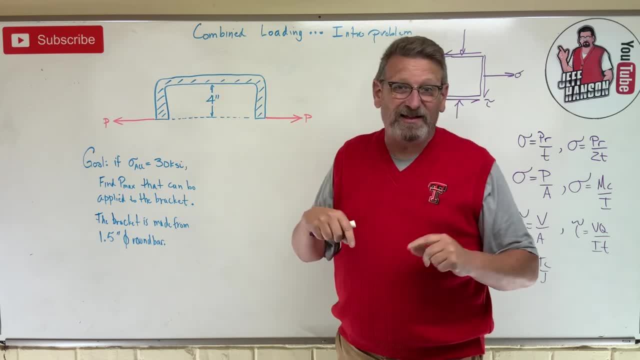 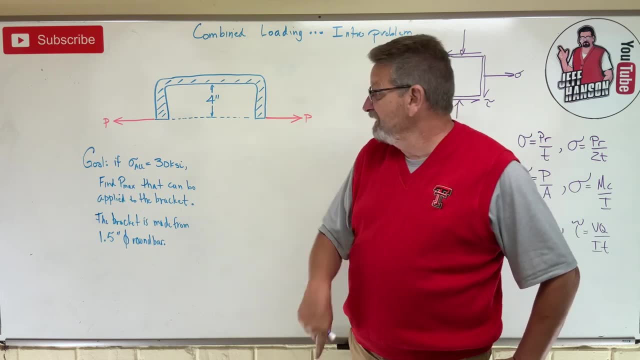 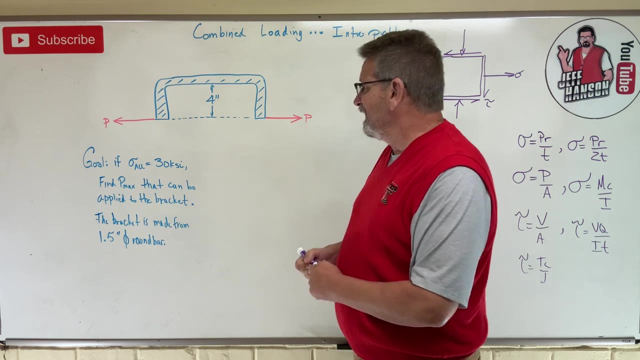 you. you need to go back to my statics lectures, way back, and you need to watch the very first statics lecture again. okay, It'll explain to you why that the force on that bar is only 1P. okay, Think of it like: 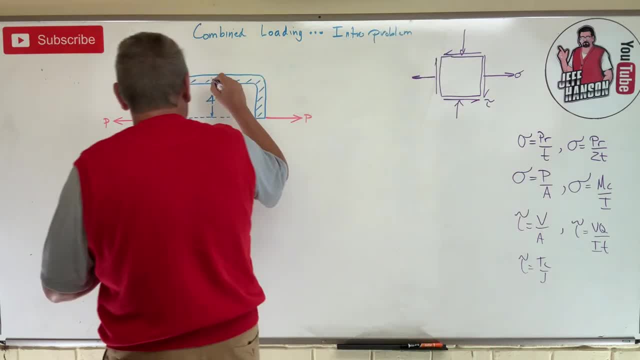 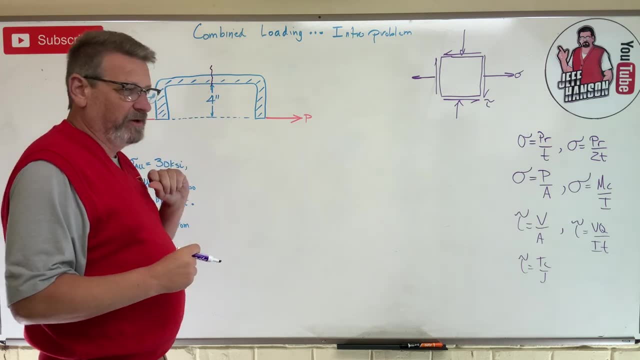 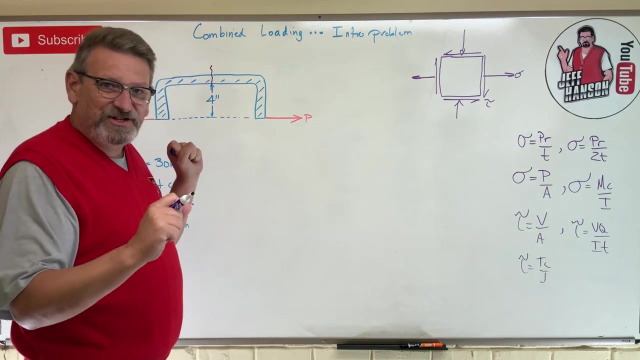 this: okay, We want to come in here in the middle of this bar and we want to look at what's going on right there in the middle of that bar. okay, There's two things going on in the middle of that bar. Number one, as I pull on this: that bar is getting stretched. 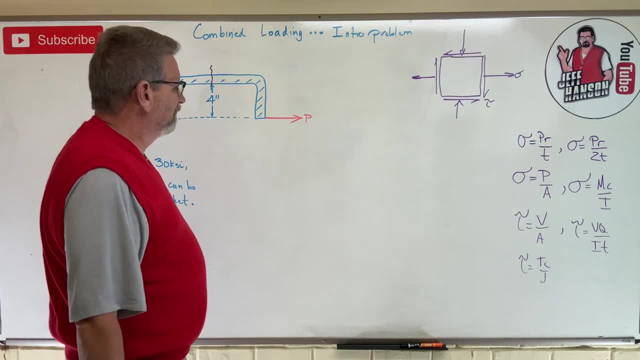 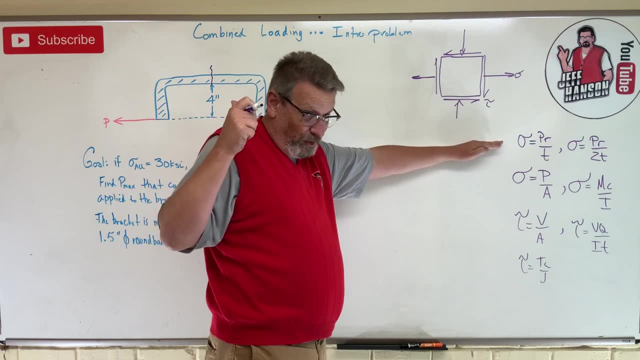 isn't it? Now, what does that sound like? Are we going to have any kind of PR over T or PR over 2T? Is that bar, that solid bar? is it a pressure vessel? No, So there's nothing happening there, But we do have just P over A. 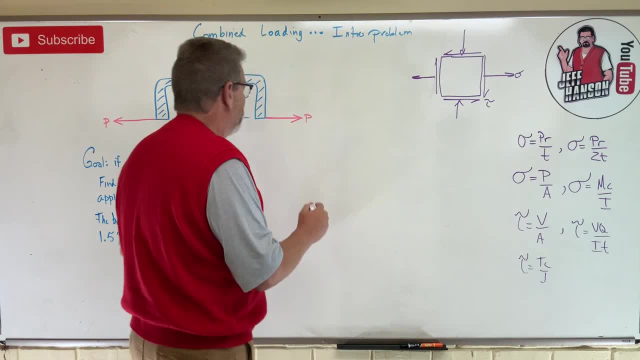 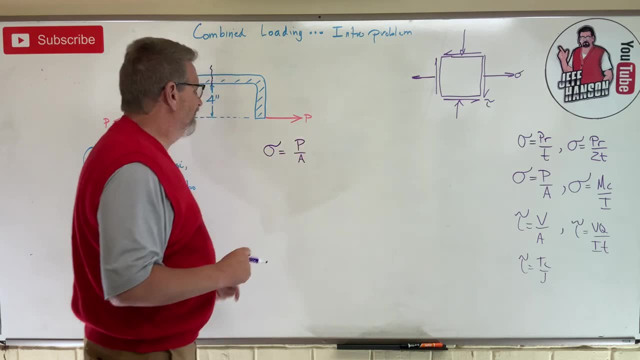 don't we? That's the sigma stress from just getting stretched. okay, So what we have is sigma is equal to P over A. okay, It's stretching me. okay. Now do we have anything else? Do we have MC over I for sigma? Do we have MC over I for sigma? Do we have MC over I for sigma? 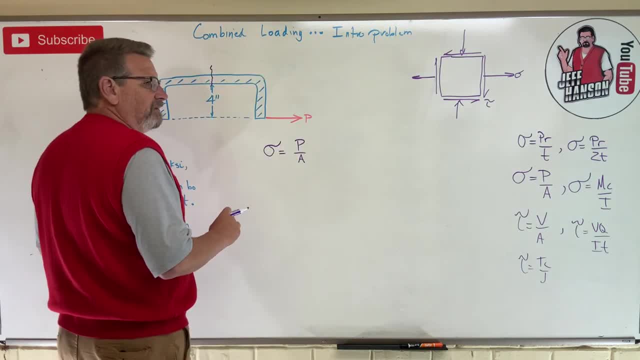 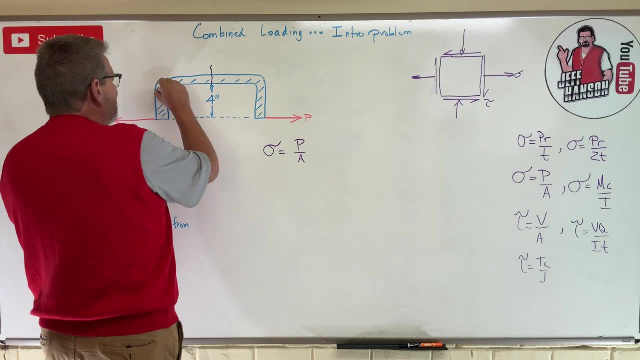 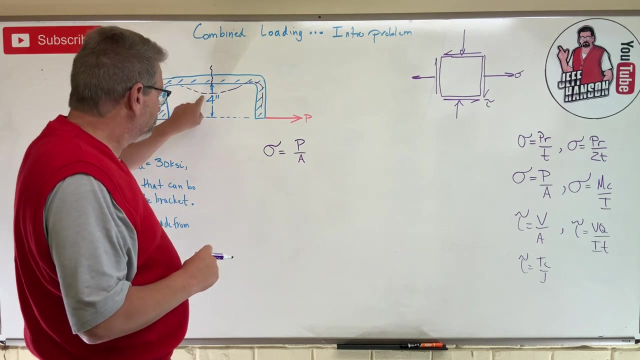 Well, the answer is yes, we do, Because, look as I pull on this, these two ends want to stretch out and it makes this guy kind of want to do this in the middle, okay. So it makes it want to bow down, okay. Now what happens here is that the top is in compression. 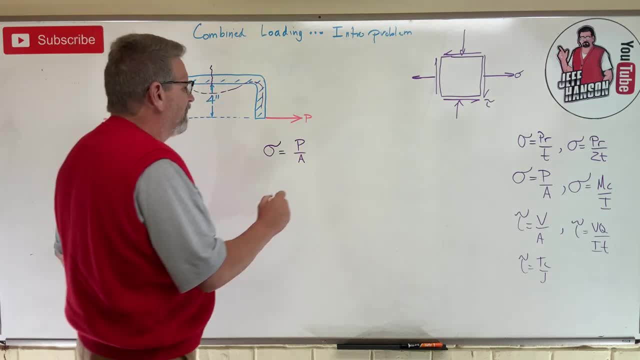 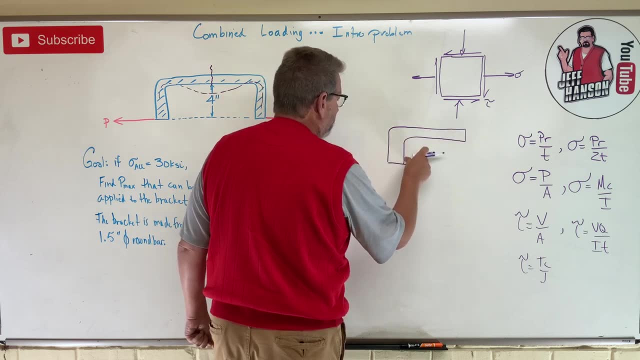 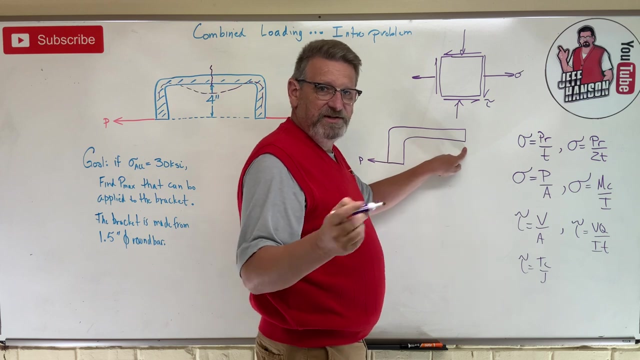 and the bottom is in tension. Now I'm going to cut this in half, okay. So if I cut this in half, number one, I get this. Okay, And here's the force P. Then what's over here on this side, Every time you cut, 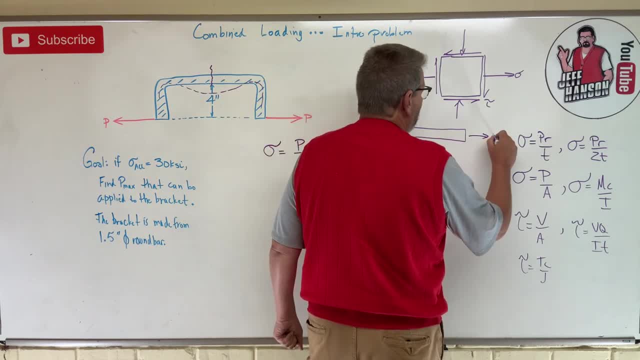 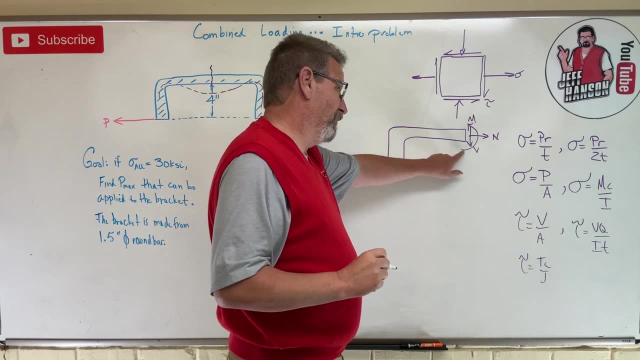 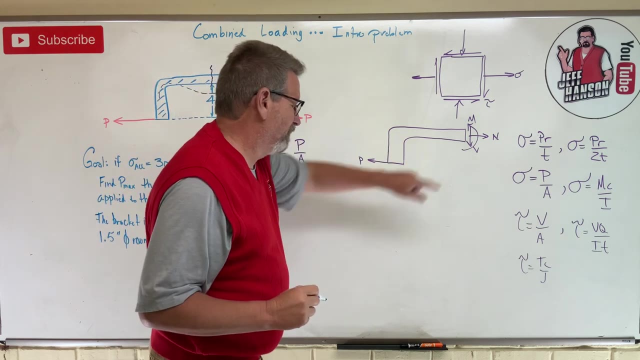 the P you must have. what do you have in V? okay, Those are those internal forces, right? That's the M that we need. That N is this guy right here? Well, he's equal to P, isn't he? Sum of the force of the X? that guy's got to be equal to that guy. V- how many forces? 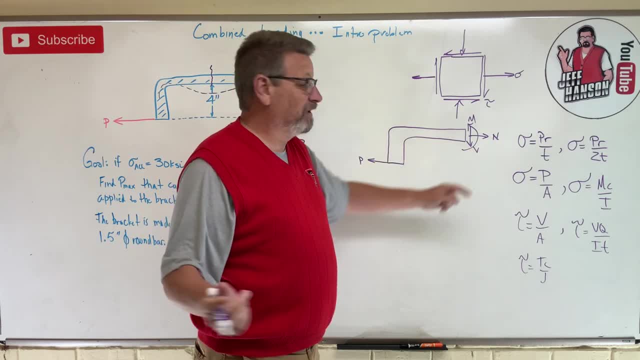 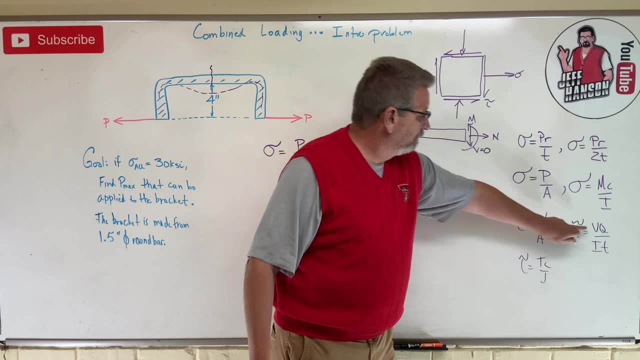 in the Y direction. do you see in the Y direction? How many forces in the Y direction do you see in this problem? Zero, V is zero. So if V is zero, what does that mean? There's no shear stress in that part right there. None, okay, No shear stress. So all we're calculating: 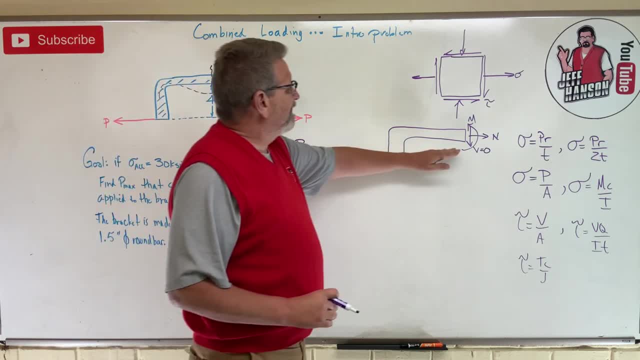 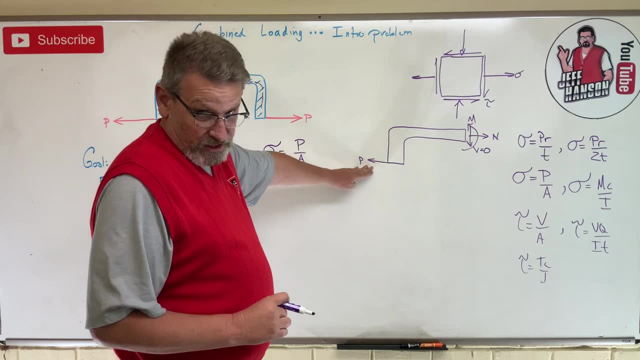 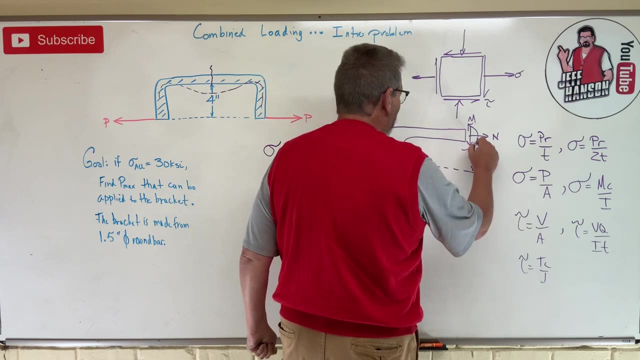 is sigma stress, But is there a moment? Well, look, there's a force in the X, so I'm going to need a distance in the Y, right, Yeah, yeah, yeah, Y'all remember the song. Don't make him sing the song, please, Okay. 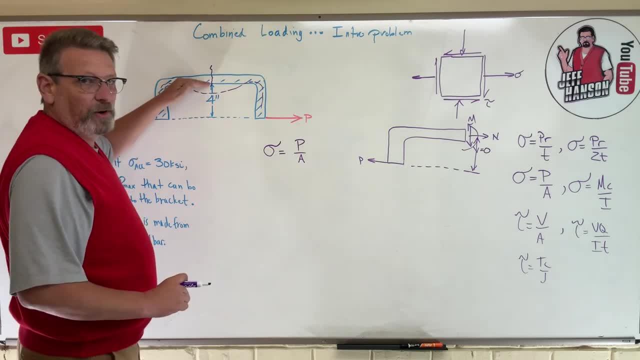 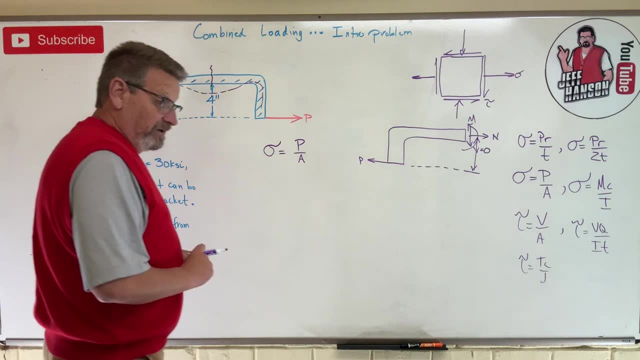 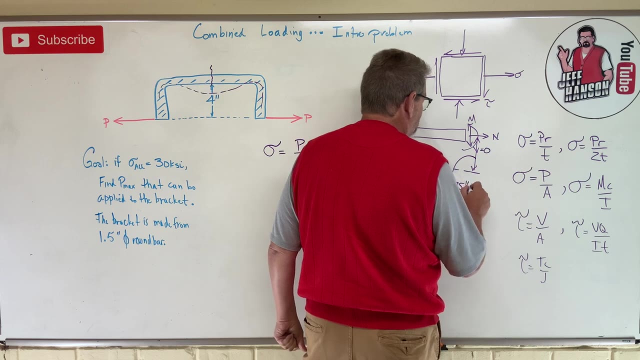 So this is what is this. It's four inches to the bottom of the part, plus I need to go to the middle of the part, I need to go to the centroid. So four inches plus it's an inch and a half diameter: 0.75.. So this is this. here is 4.75 inches, isn't it Okay? 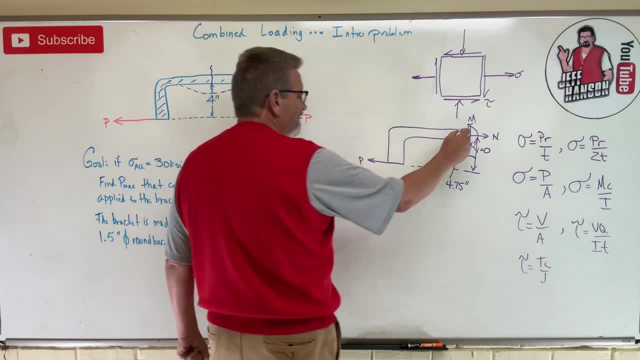 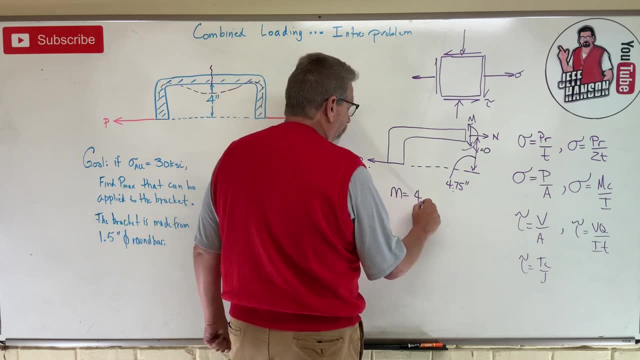 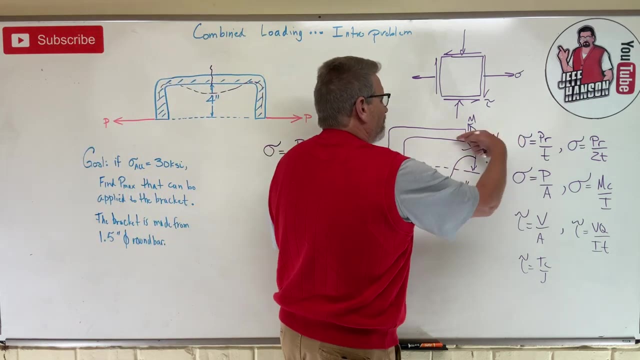 So how big is that moment? right, How big is this moment? Force times distance, that's the force, that's the distance. The moment is equal to 4.75 P. okay, Now it's causing bending. Let's look at this end where I cut that. Let's look at it straight on. What does? 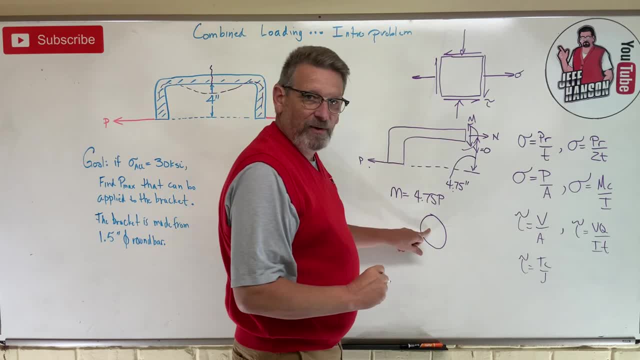 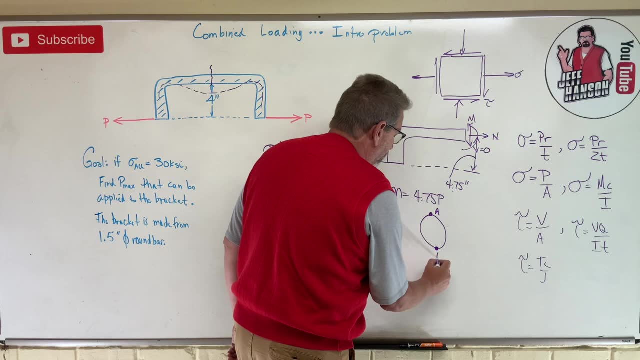 it. look like It. looks like that. okay, It's a piece of round bar. Now. there's a piece of material on the top, we'll call him A, and there's a piece of material on the bottom, we'll call him B. okay, Now he's being bent right with MC over. I. 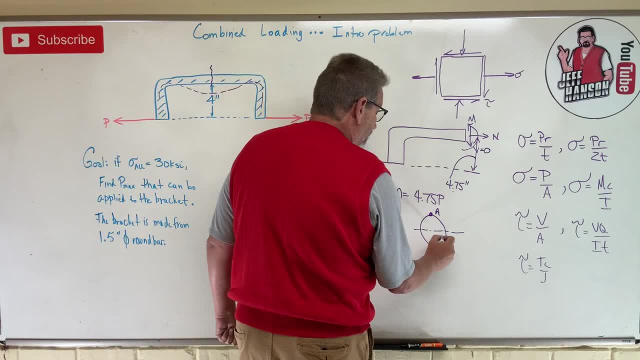 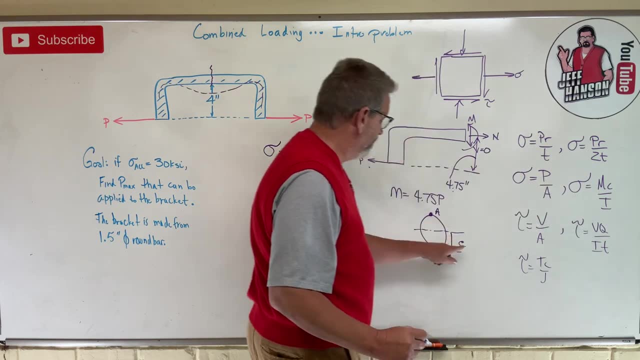 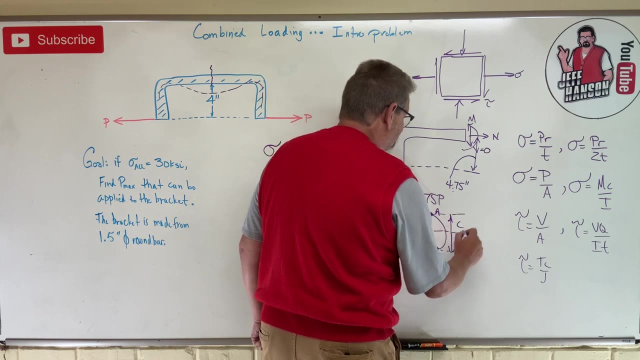 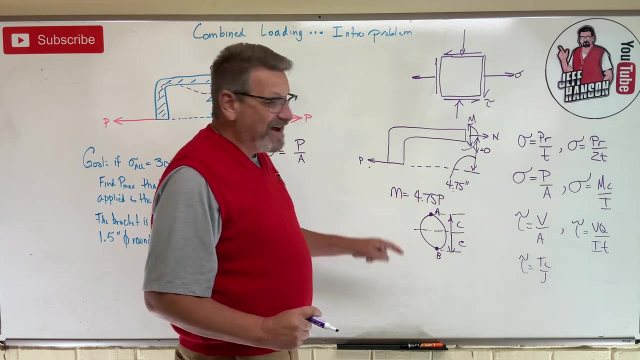 Here's the neutral axis, okay, And guess what? This is the distance C in my MC over I right for point B. And this is the distance C in the MC over I equation for my point A: material right. We're asked to find, though, what are we asked to find? The max, the biggest, okay. 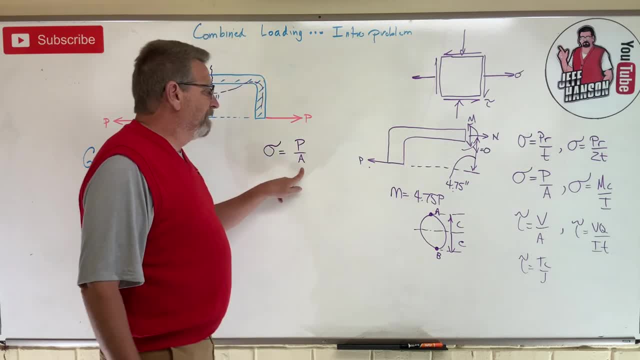 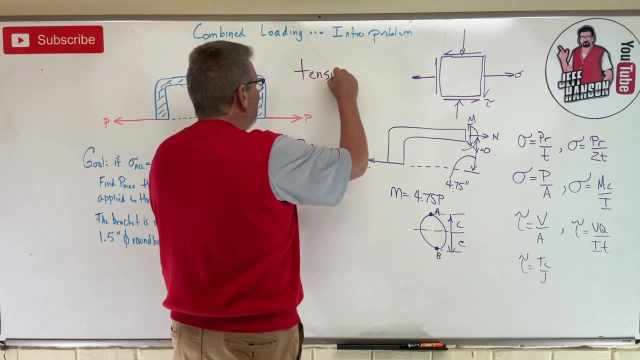 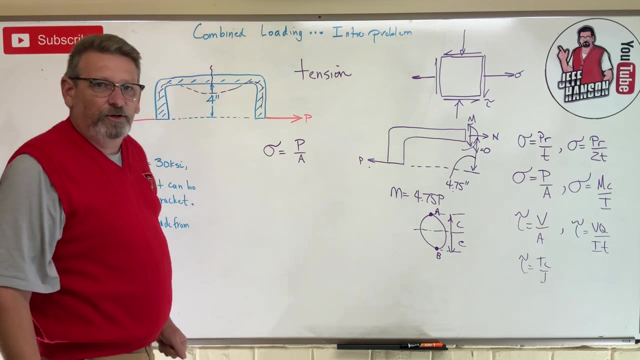 Now, P over A. Remember, tension. what does tension start with? A positive sign, That's right, okay, Tension starts with a positive sign. So, as I'm pulling on this bracket, ugh, am I making it longer or shorter? Longer, Yes, that means it's a positive P over A, because 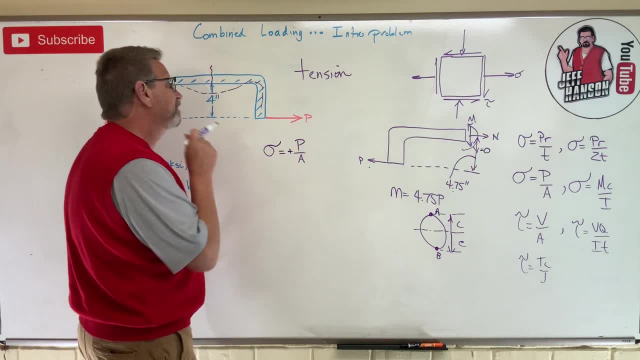 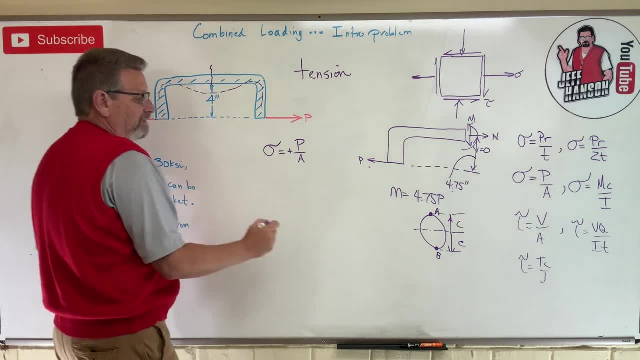 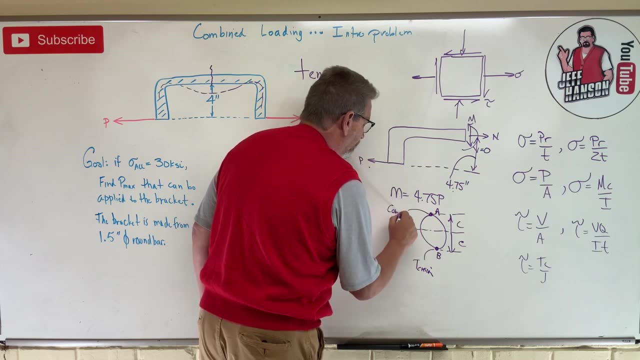 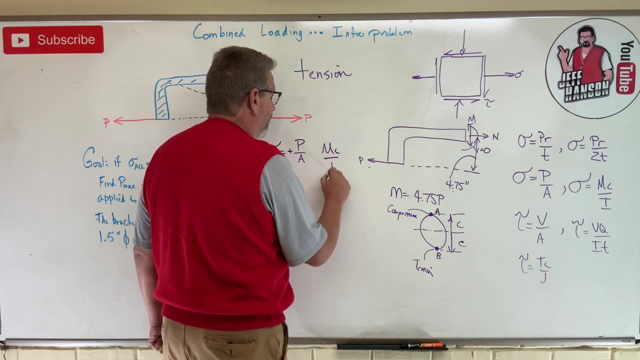 The other side is in compression, The other side is in tension. So down here we're talking tension and up here we're talking compression. okay, So here's what I have: I have P over A stress, but I also have MC over I stress. okay. Now, if I'm talking about point A, the 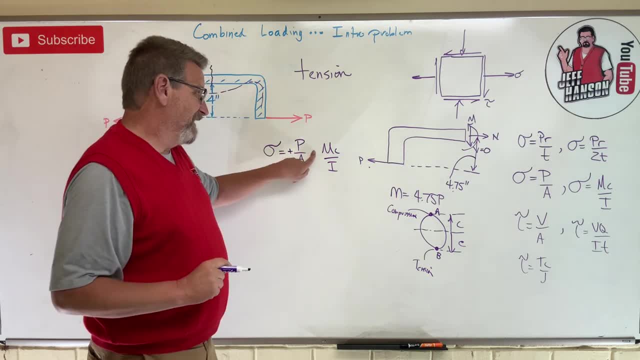 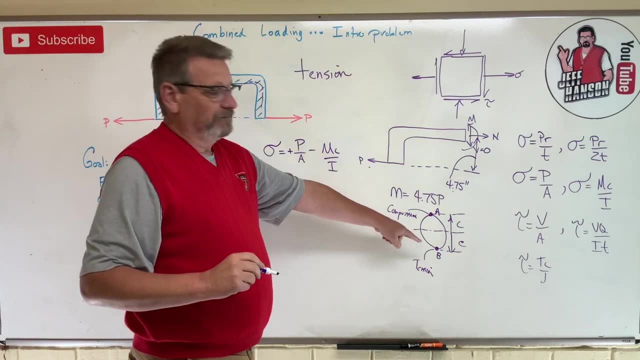 MC over. I stress, he's in compression. that sign's going to be a negative. okay, So I'm. But if I'm talking about point B, down on the bottom, the stress down there is going to be in tension, so it's going to be a positive. 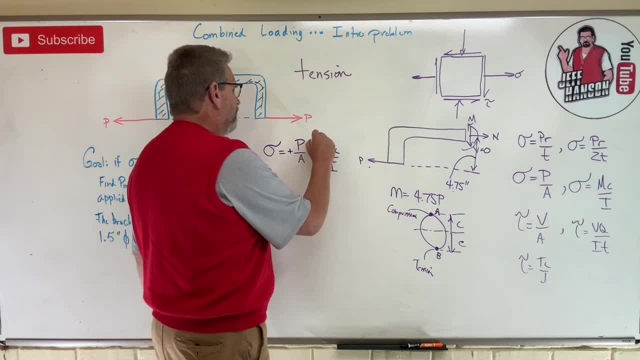 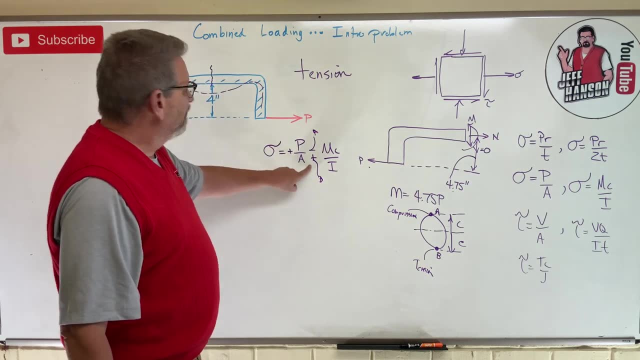 So which one of these conditions do you want to go with material A, or do you want to go with material B, right on the top or on the bottom, to make the max, the worst case, the worst sigma stress? Well, we're going to have to go with one with a plus right. 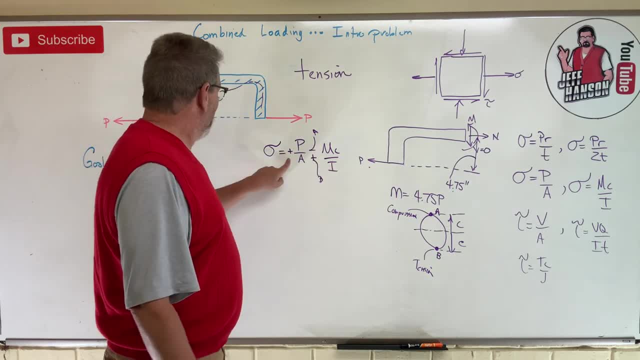 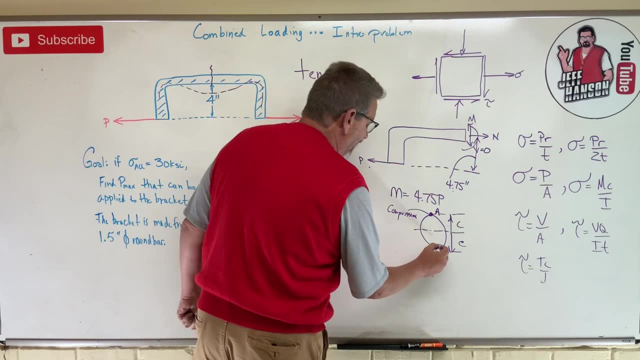 Plus and a plus make the biggest number right: A plus and a minus, not the biggest number. okay, So the max is occurring down here, at point B, on the very bottom of this part. It's down right there, right on the bottom of that part. 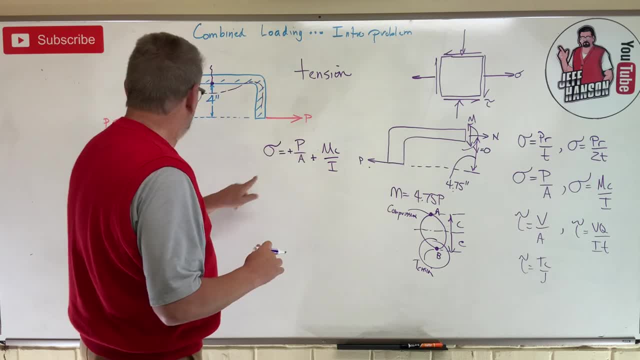 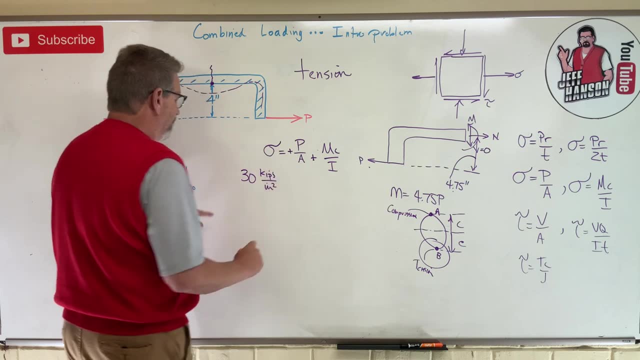 And here we go, Let's calculate what it is. So on this side, we have what? 30 kips per inch squared, That's our sigma allowable, okay. Okay, It's equal to P over A. Guess what we're trying to find? 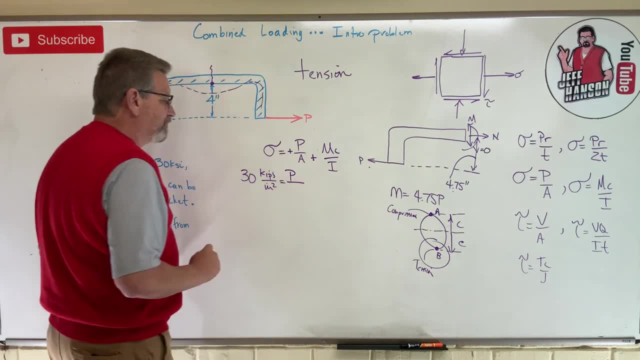 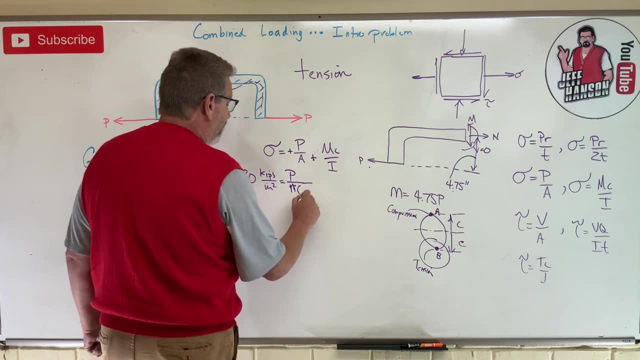 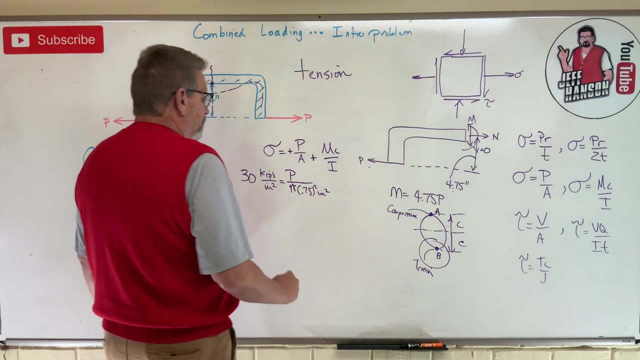 We're trying to find P And the cross-sectional area. what's the cross-sectional area there? That's just pi times R squared right, So 0.75 squared and that's inches squared, okay. So look, that's in kips over inches squared. 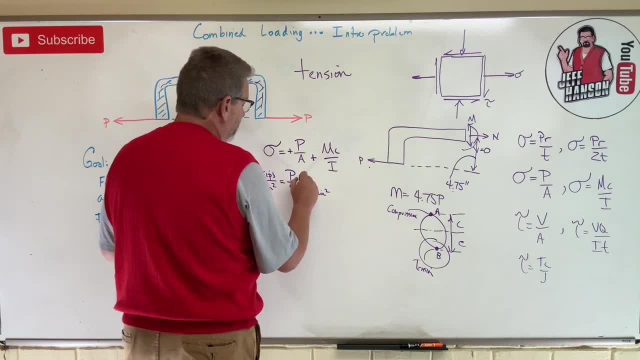 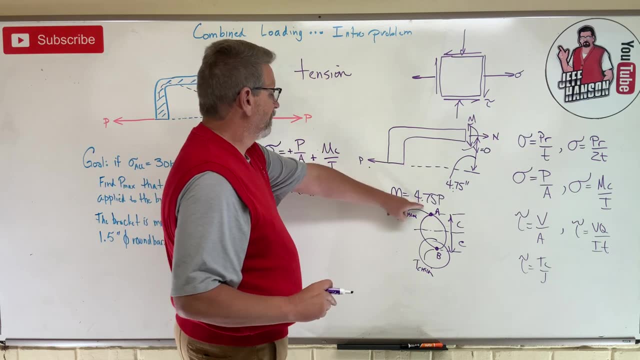 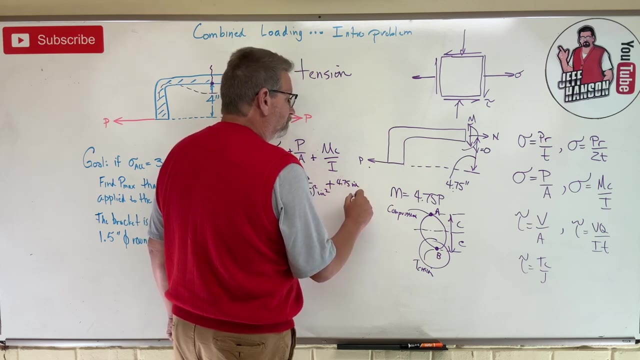 P is in. what's it going to be? That's going to be in kips, okay. Plus now I've got MC over I. What's M 4.75 inches and what is that unit in Kips, right? 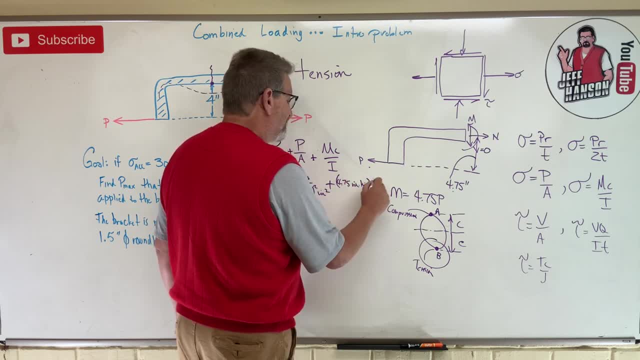 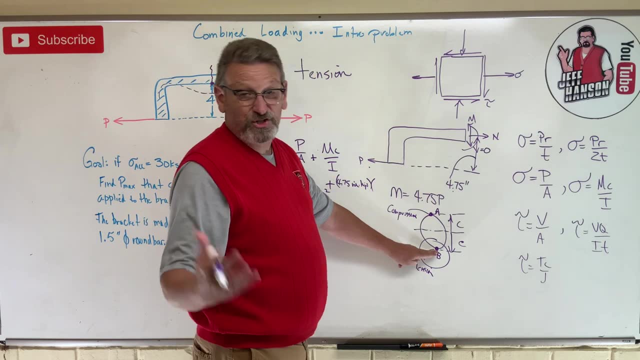 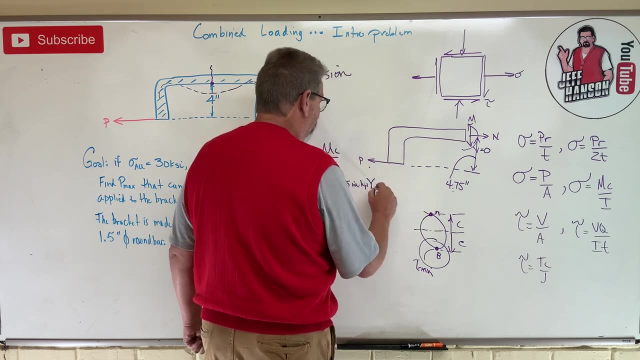 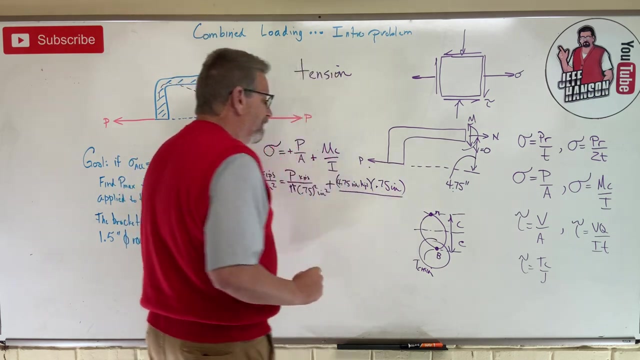 Inch kips times C. What is C? C is the distance from the neutral axis to the outside of the part, which is just a radius, in this case Right, And so C is going to be 0.75 inches. So I've got inches squared on the top, divided by I. 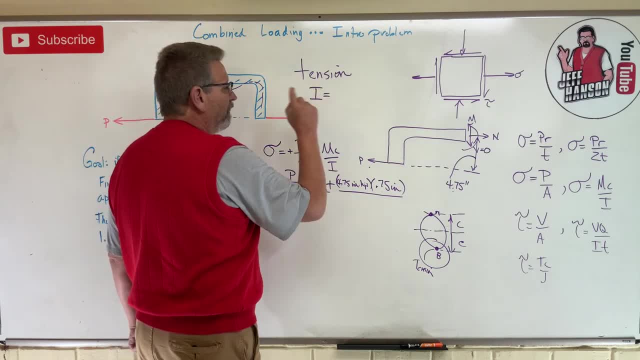 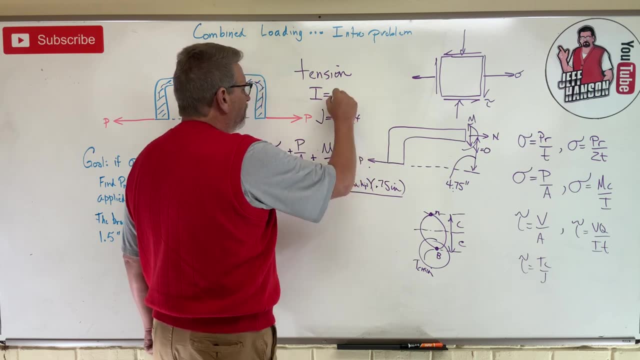 Uh-oh, What is I for a round part? Now, don't get this confused with J, Do you remember J? J is pi over 2, C to the fourth. I is pi over 4, R to the fourth, okay. 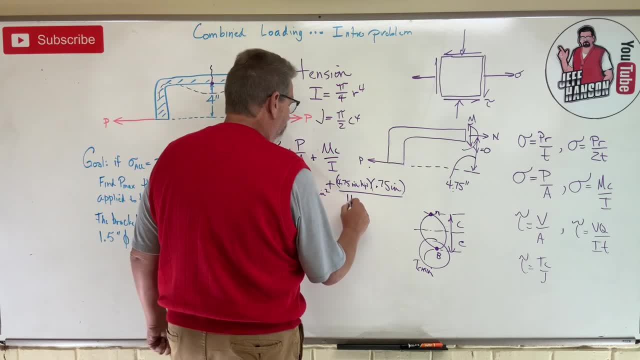 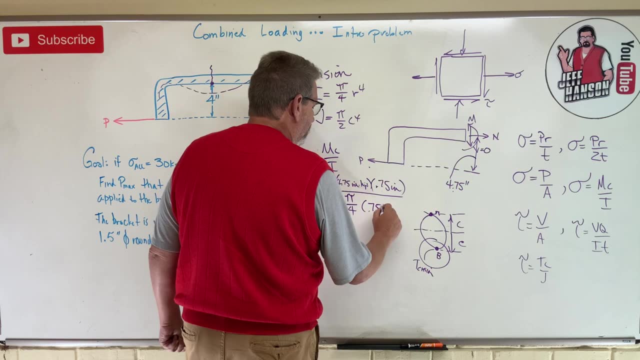 So we're going to use this guy up here. So we're going to use pi to the fourth Or pi to the fourth, Pi over 4,- sorry times- 0.75 to the fourth And that's going to be inches to the fourth. 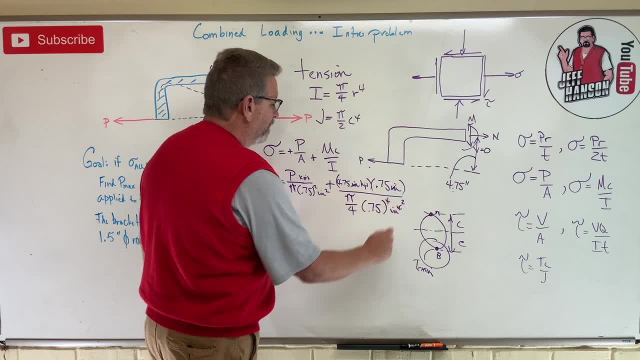 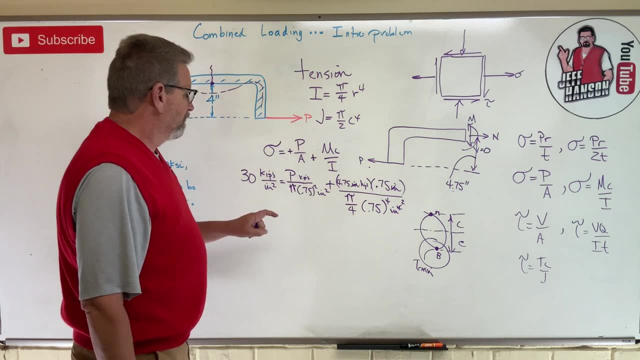 So guess what? These two inches. I'll cancel that with 2.. So this one has kips over inches squared, This one has kips over inches squared, And this one has kips over inches squared. So what do we have? 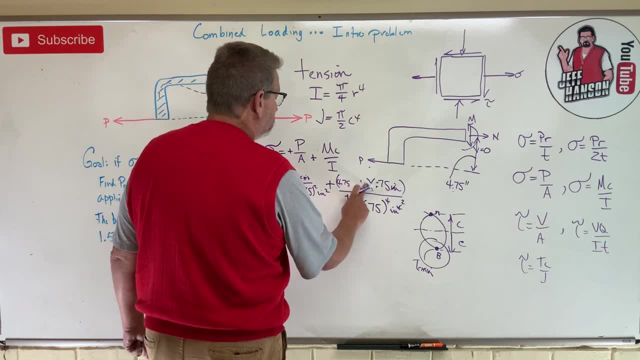 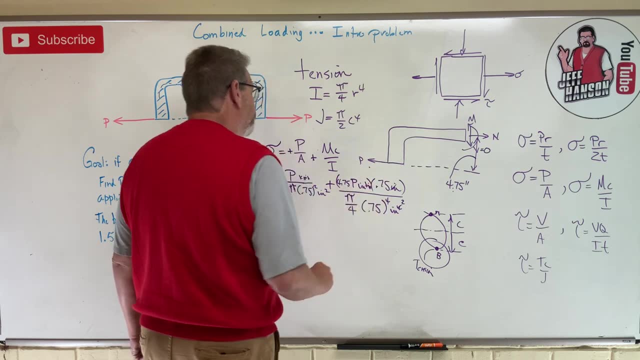 Oh, you know what, Dr Hanson, You left out pi? It's 4.75 pi inch kips. okay, So we're looking for this pi, aren't we? Let's see if we can find it okay. 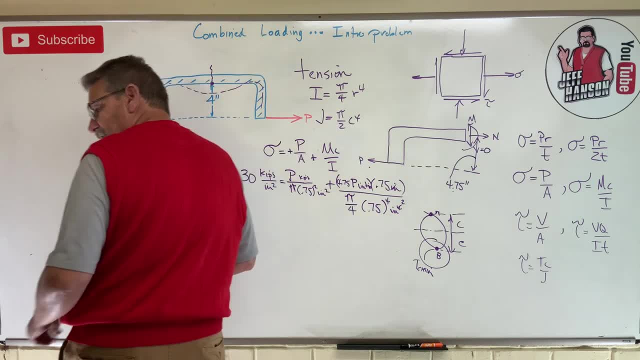 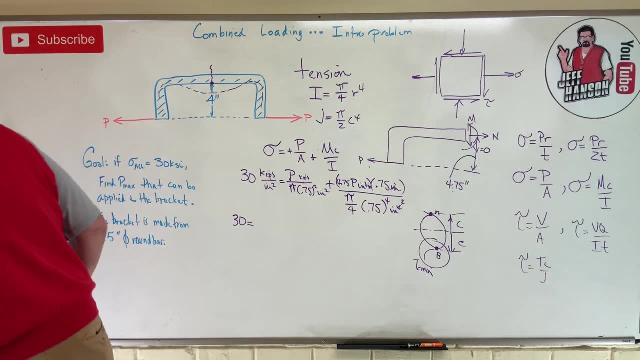 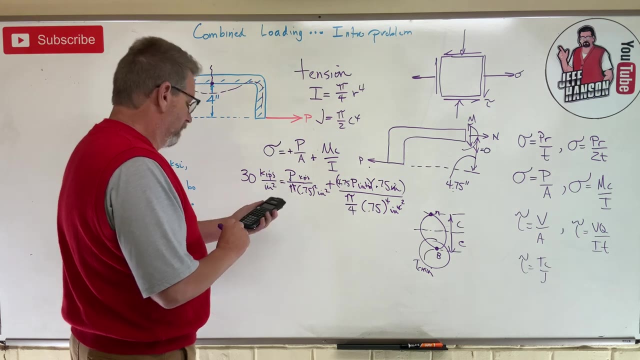 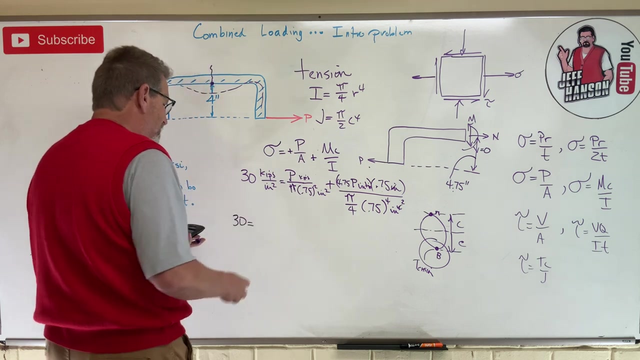 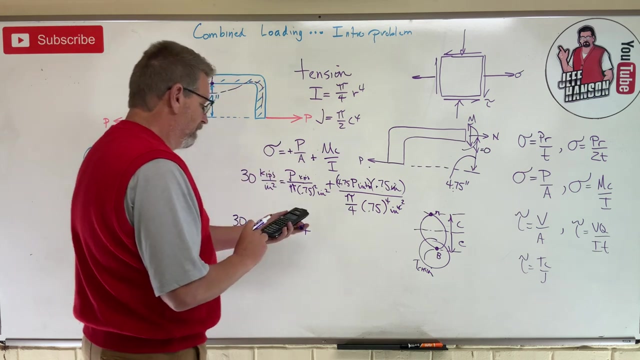 So 30 is equal to calculator. Okay, Ooh, that calculator didn't come on. How about this calculator On? Okay, so what do we have here? 1 divided by pi, divided by 0.75 squared is equal to 0.566, 0.566p plus. okay, what do we got over there? 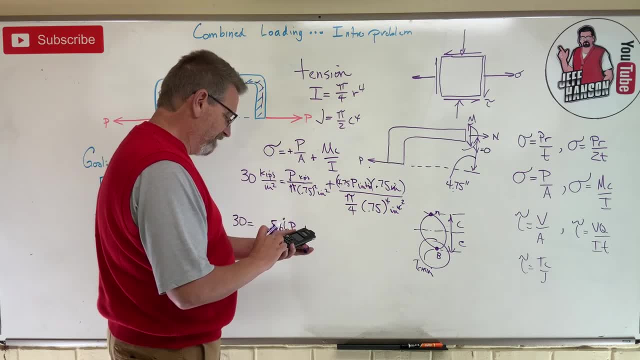